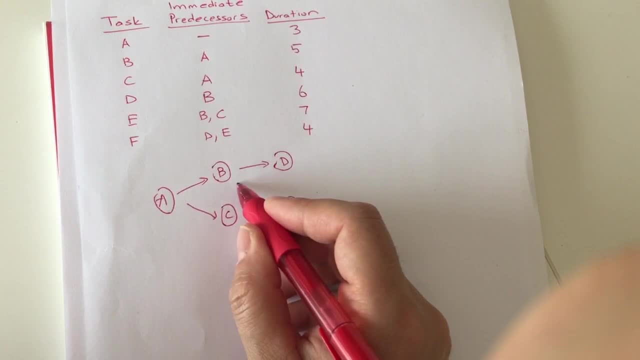 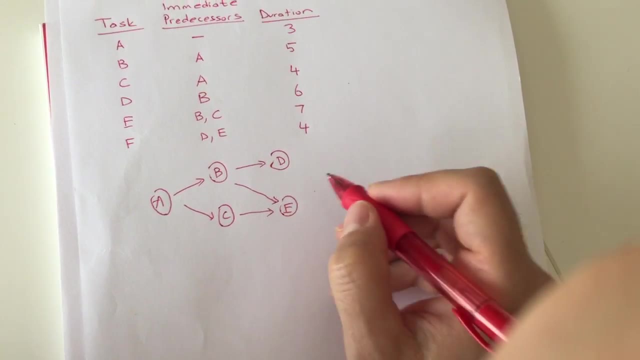 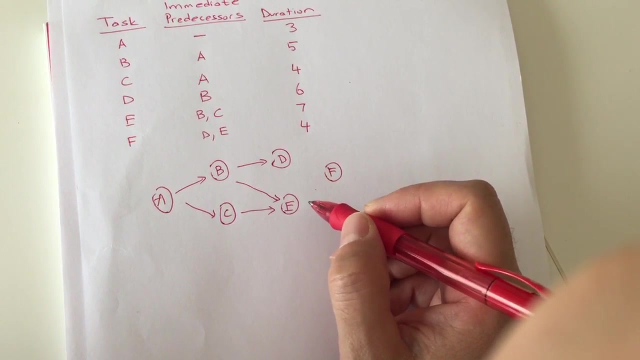 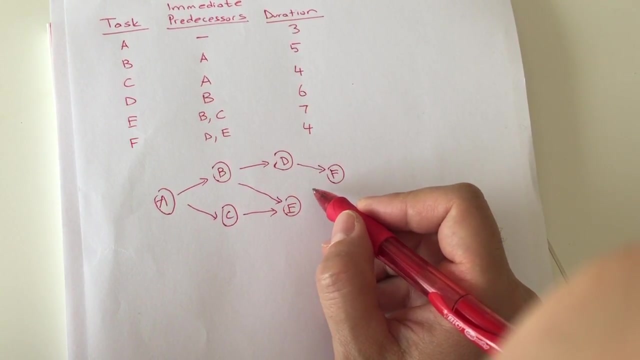 them. so in that case I'm gonna put E here. I will make an arrow from B and also an arrow from C that goes into E, and then I have F, and F has two predecessors. so two tasks have to be completed before F can start, and that is D to F and then E to F. then what I will do is I'm going to put 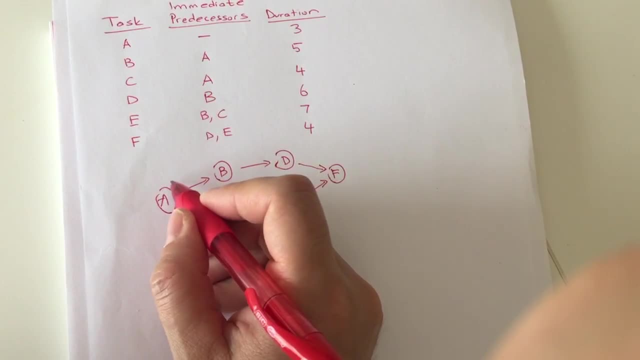 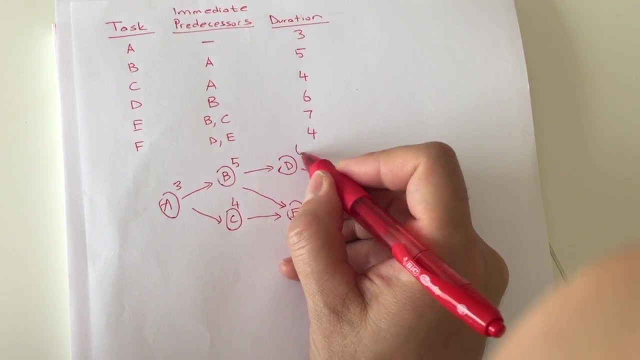 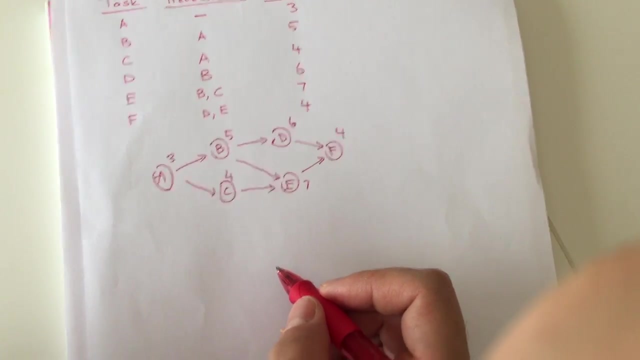 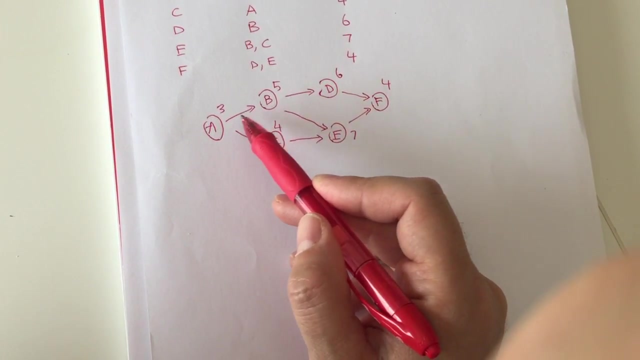 the durations of each task on top of each one of them. so three, five, four, six, seven and four. so that want I have to do is I'm going to take a look at the the paths that goes from A to F. remember that whenever there is a relationship, 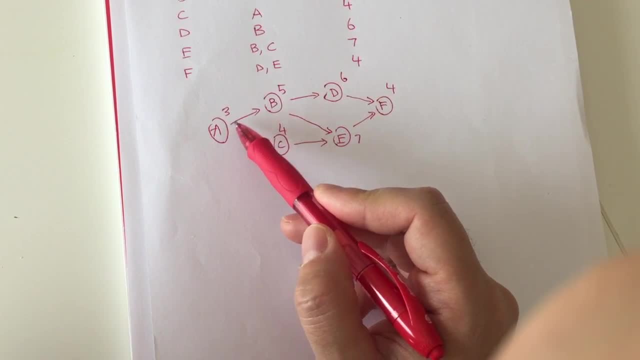 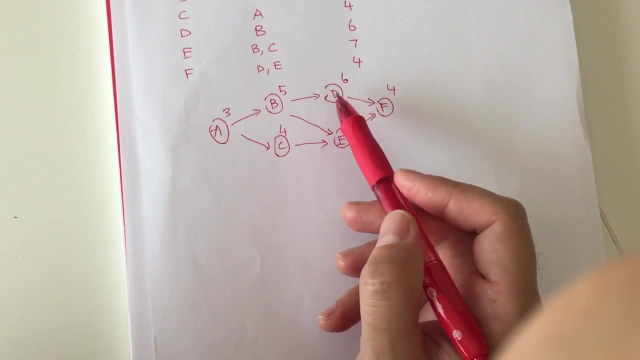 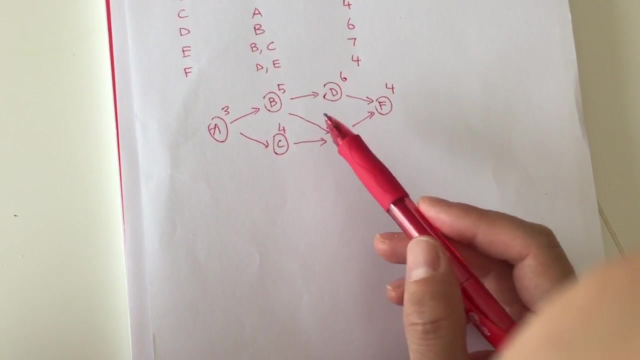 between each activity. you have to complete the activity first, and then the task has be completed first. that's the first step, next activity after. so, for example, if I need to do D, I have to finish A and B. if I need to finish, let's say, E, I have to finish ABC together. then I can just 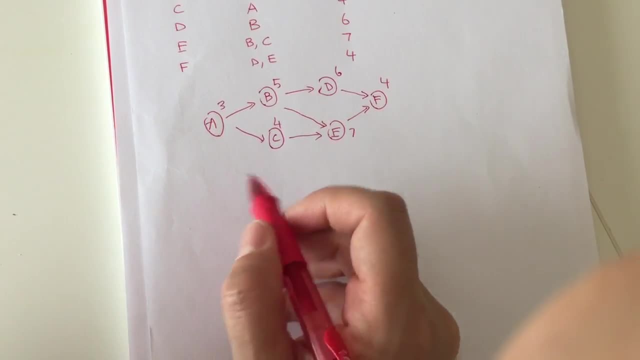 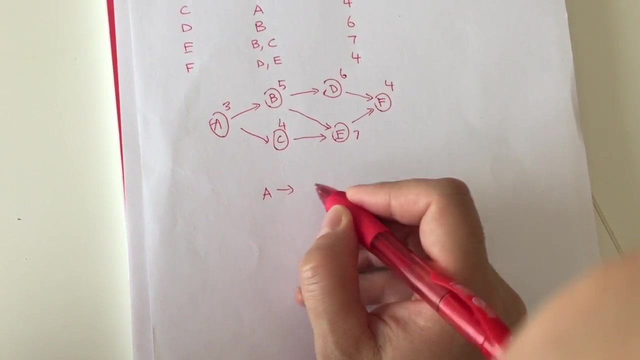 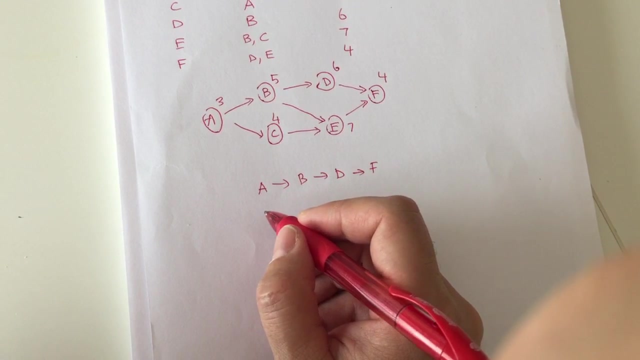 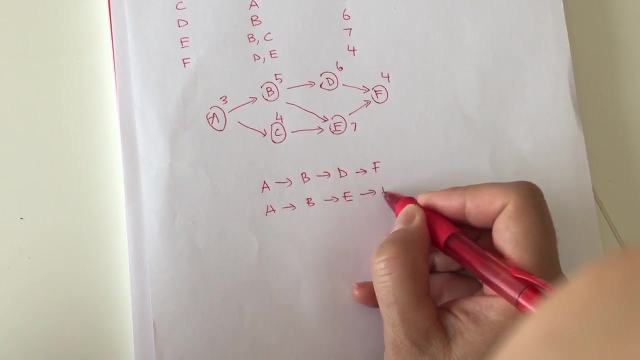 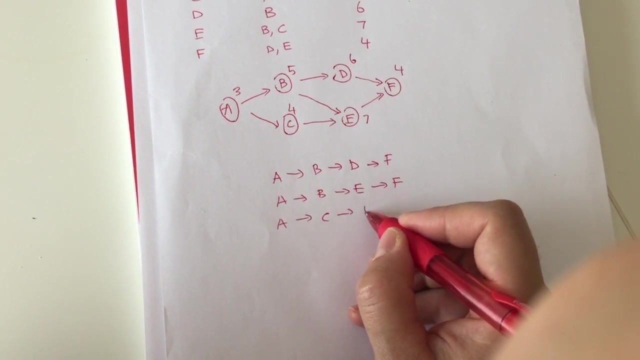 start E. so what I need to do is I'm gonna put all the paths that are coming from the beginning to the end, so that I have A to B, to D to F, and then I have another path that goes from A to B, then E to F, and the third path is A to C to E. 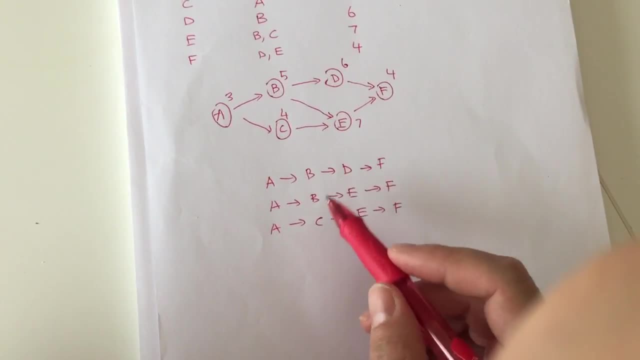 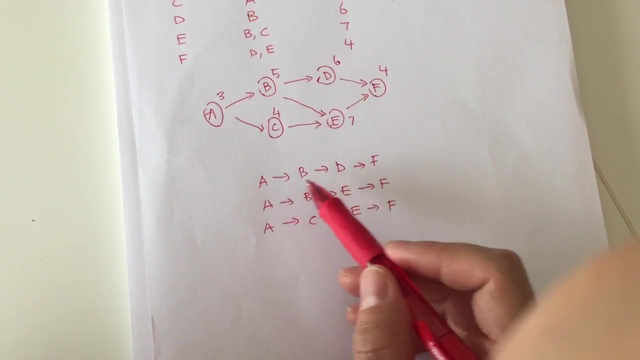 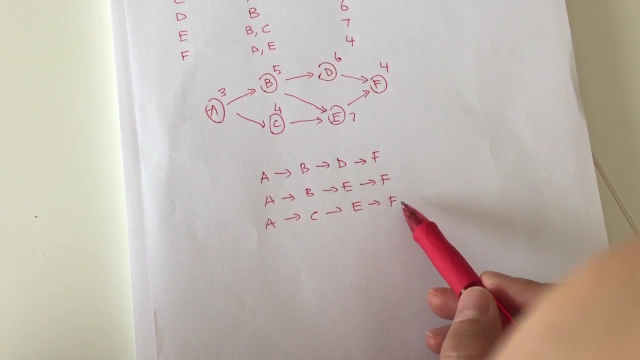 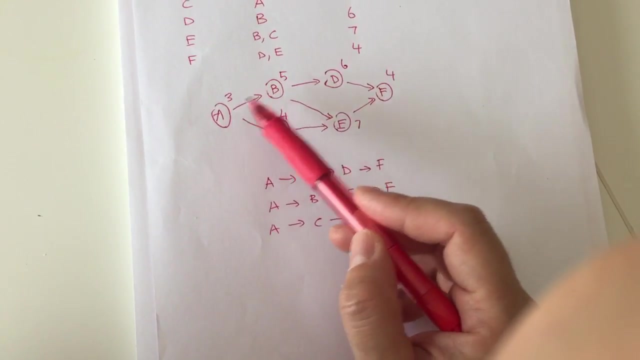 to F. what I did is I outlined all the paths that are going from the beginning to the end. so I have to complete this paths in my project and whichever takes the longest time is going to determine my project duration. so ABD F is 8 and 10. 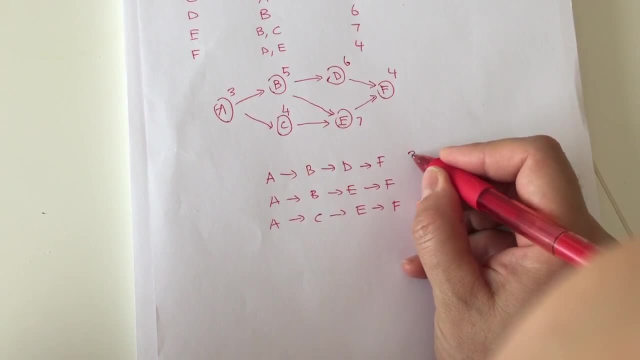 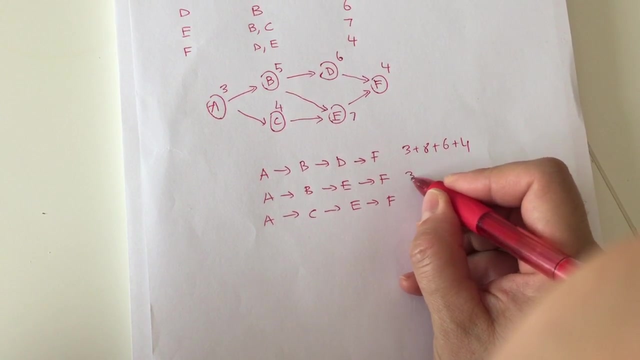 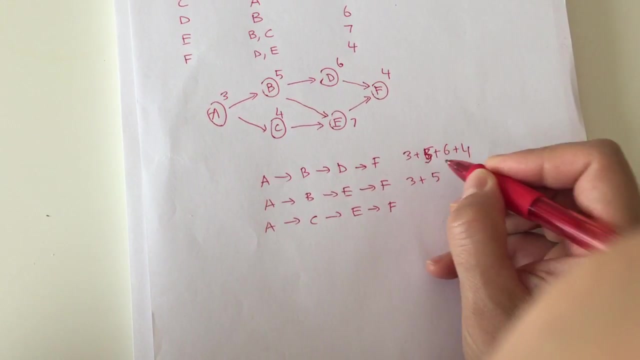 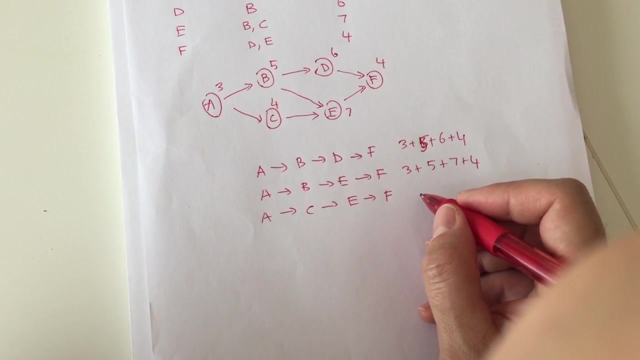 here, which is 18, so 3 plus 8 plus 6, six plus four, and a, b, e, f is three plus five plus- i made a mistake here- three plus five here. okay, so three plus five plus seven plus four. and the third path is three plus four plus seven. 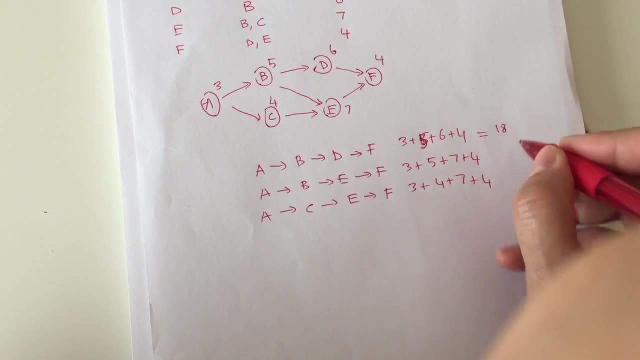 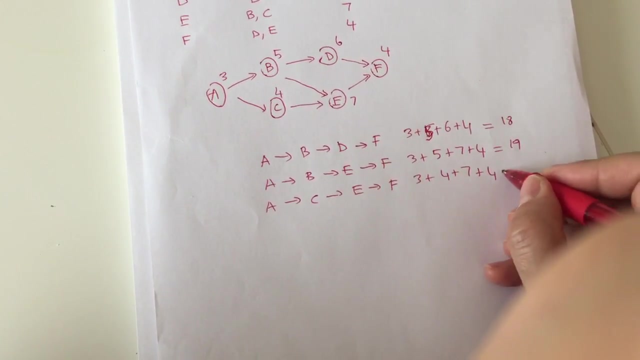 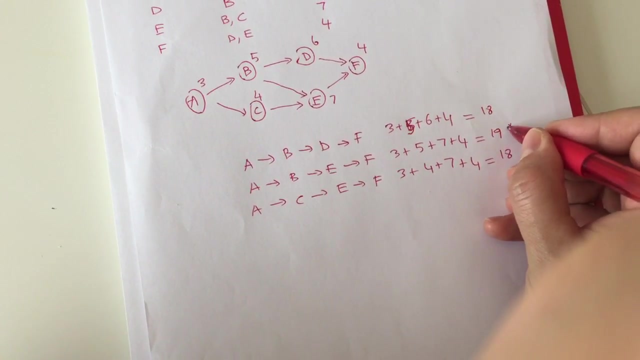 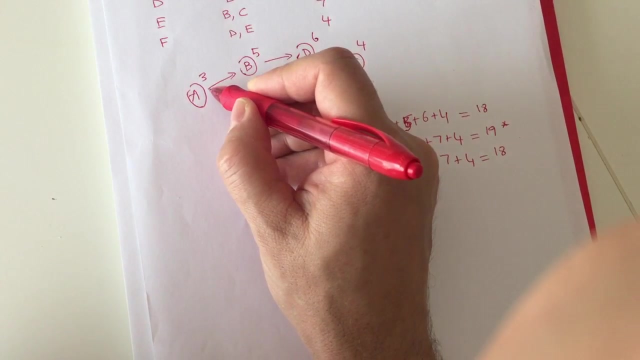 plus four, so the total is 18, and this total is 8, 7. 15 plus 4 is 19, and this total is 7 plus 7 is 14, plus 4 is 18.. so i determined that a, b e, f takes the longest duration. so this is my path: a, b e, f. 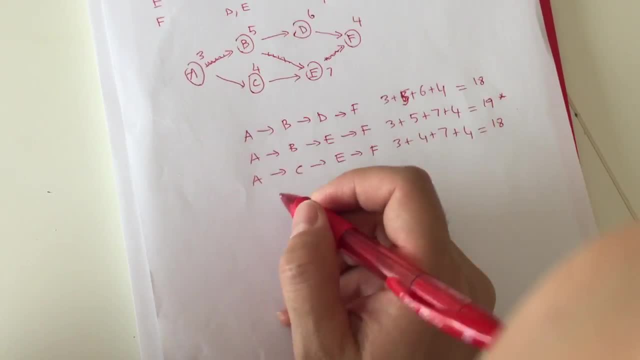 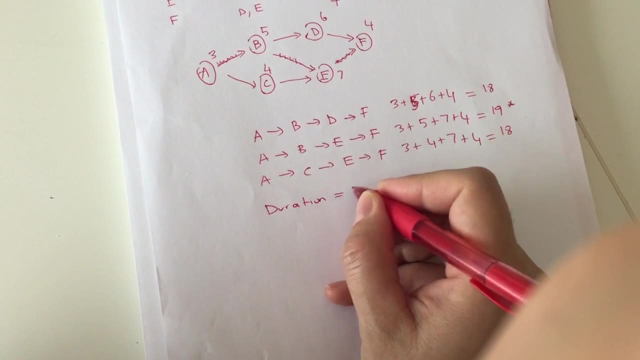 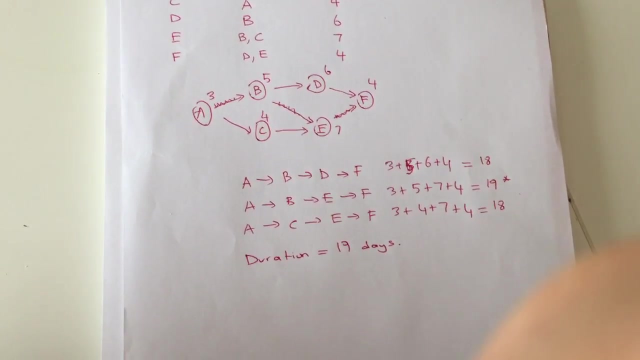 and that determines my project duration, and i'm going to say that the duration of my project is 19 days. whichever the time period is okay. thanks for watching.